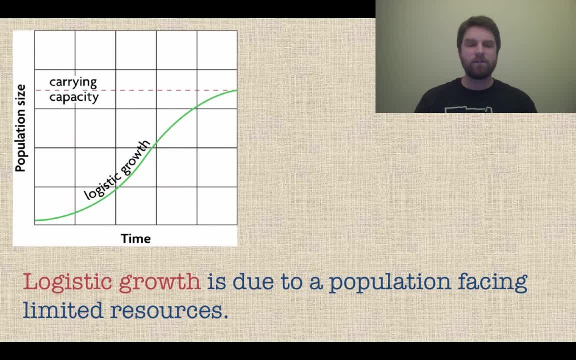 bit. So if you look at this graph right here, this is logistic growth. So you can see over time there is a period of slow growth and then there is an exponential period of growth And then the population size actually levels off towards the top there until it reaches what's known as the 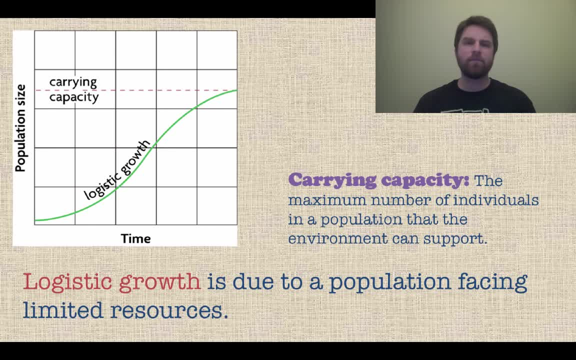 carrying capacity. So carrying capacity is the maximum number of individuals in a population that are that the environment can support. So normally populations do not go past this carrying capacity because there's simply not enough resources to handle that population. So here's another look at. 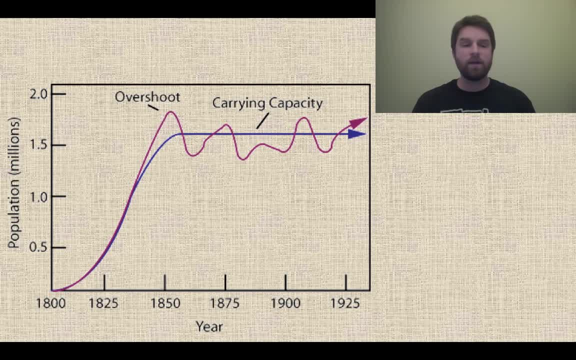 a carrying capacity curve, of a logistic growth. So you have a population that has an exponential increase in a very short amount of time and then it overshoots its carrying capacity, So some of those organisms die off. So you can see that curve going down. but then there are enough resources. 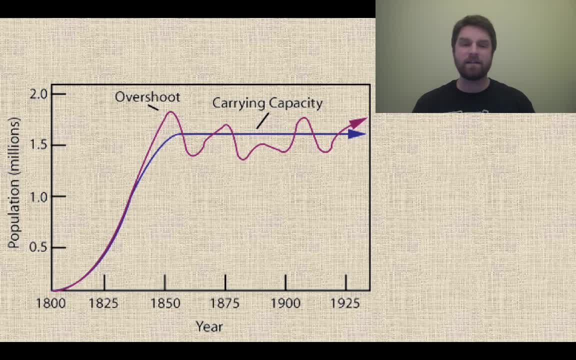 for it to come back up And every time it goes it's going to die off. So you can see that curve over that carrying capacity. It has a little bit of a downturn until it kind of averages out to that carrying capacity which looks like it's just over one and a half million of whatever this organism. 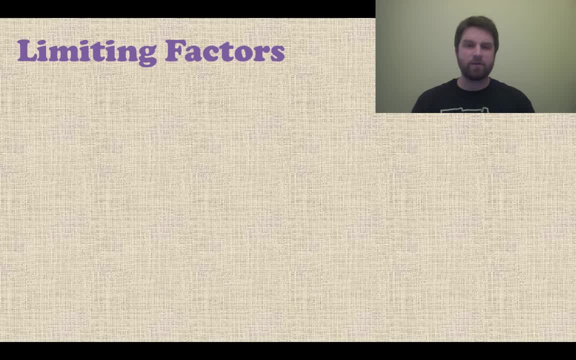 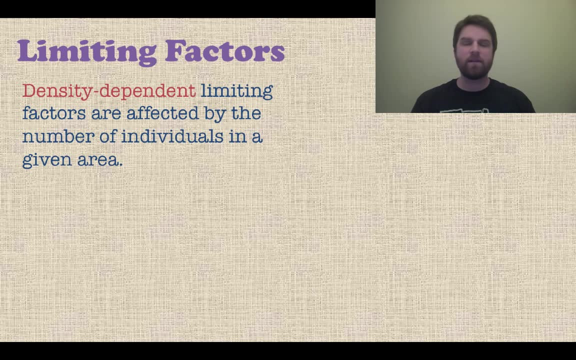 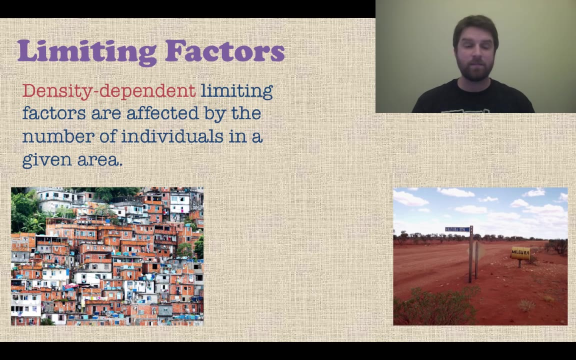 is. So now let's look at some limiting factors for different populations. First let's look at density-dependent limiting factors, And these are affected by the number of individuals in a given area, so the density of a population. So on the left you have a very, very highly dense population. 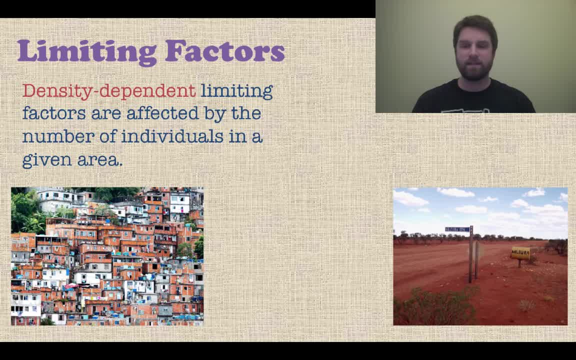 On the right, a very sparse area, so a very low density area. So these factors are things like predation. These are much more influential in highly dense populations. Same thing with competition, when organisms compete for resources. Parasitism and disease are also much more, affect dense populations a lot more. 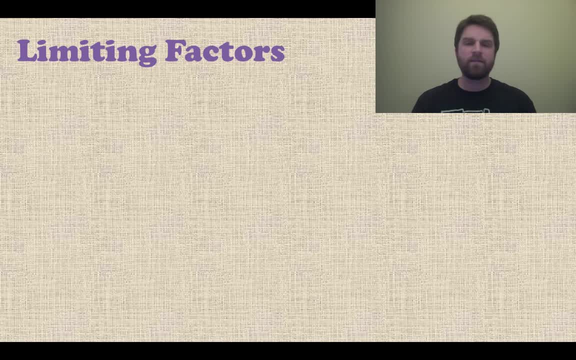 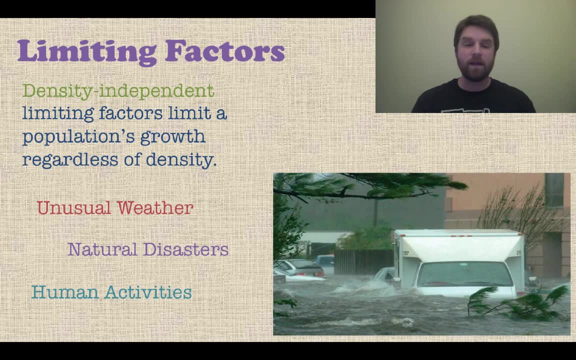 than they do less dense populations. So what are some limiting factors that are density-independent? Well, these are things that limit a population's growth regardless of its density, And these are things like weather, natural disasters or any sort of human activities, the things that we do that affect the environment. 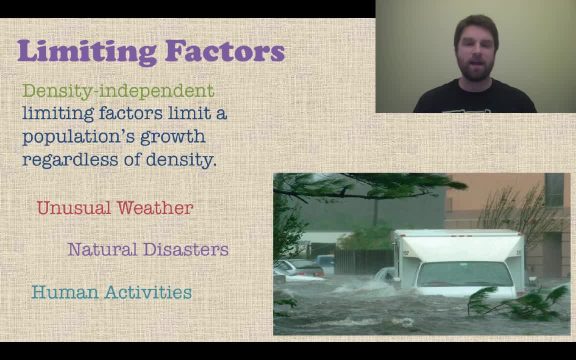 So there are density-dependent and density-independent factors. Make sure you know these very well.